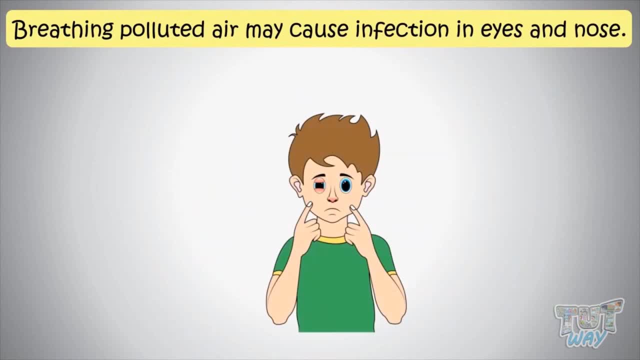 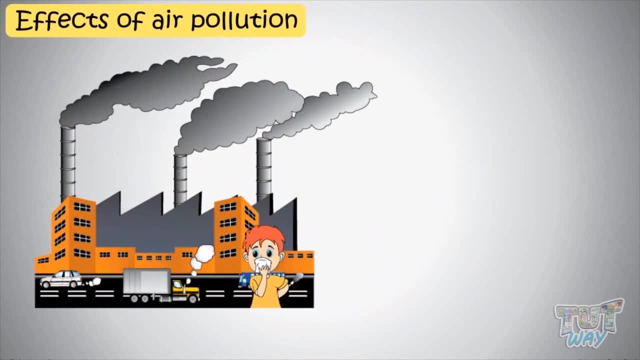 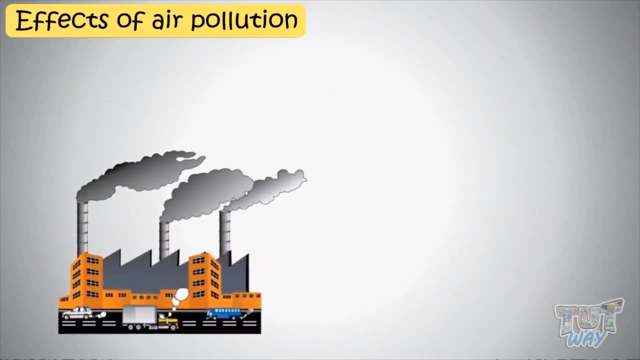 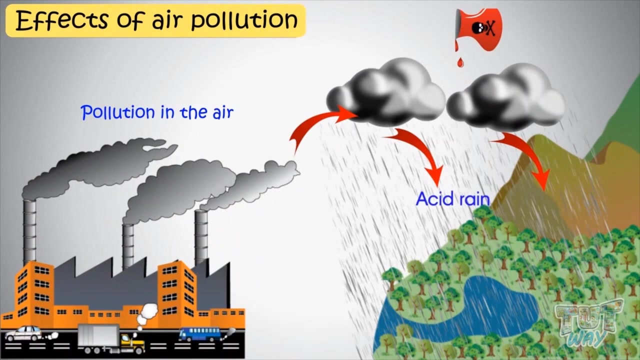 Breathing polluted air may cause infections in eyes and nose. Air pollution due to traffic is normal. This is the main reason behind the increase in number of asthma patients. Chemical pollutants in the air. when mixed with rain, it forms acid rain, which is very harmful for all living beings. 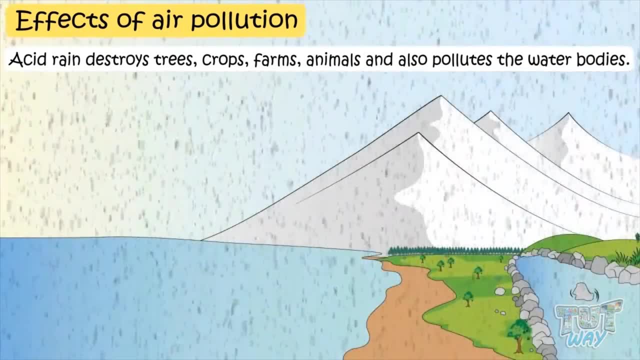 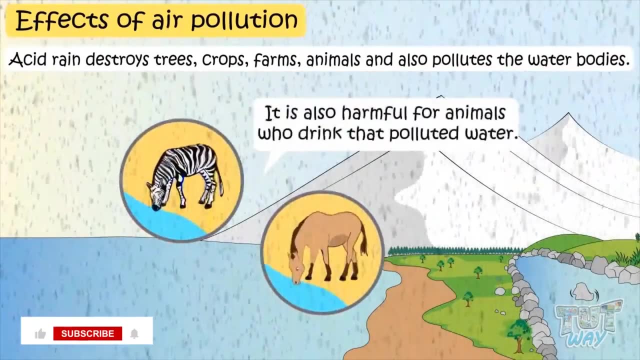 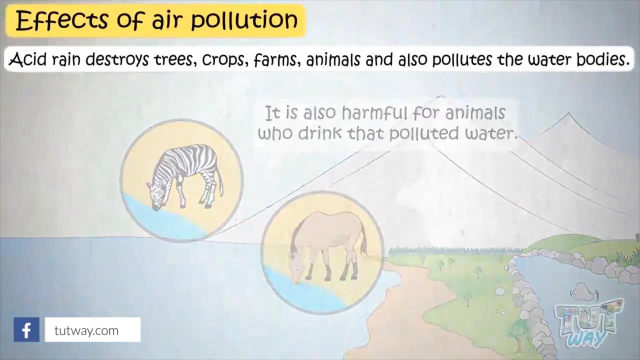 Acid rain destroys trees, crops, farms, animals and also pollutes the water bodies. that again harms the living things that depend on it. This is the main reason behind the increase in number of asthma patients. Another important effect of pollution is smog. 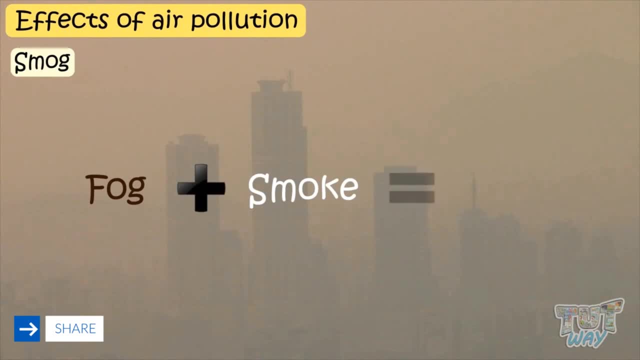 It is formed. when fog is mixed with smoke and a poisonous form of fog is formed, which we call as smog. It can be very harmful to breathe in too much of smog, as it contains a pollutant called ozone- An ozone. 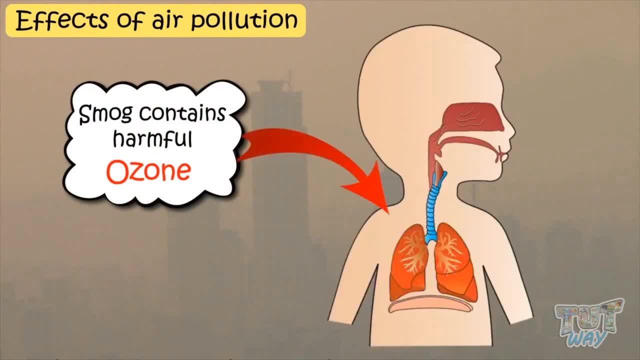 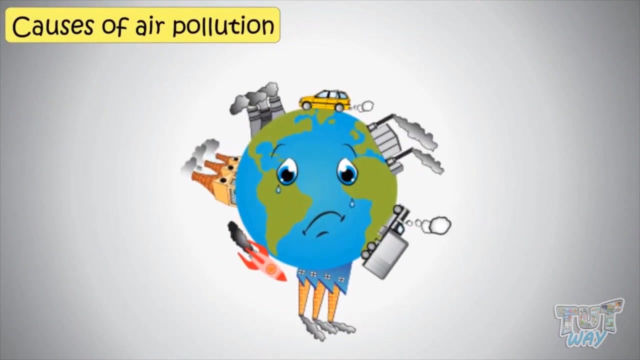 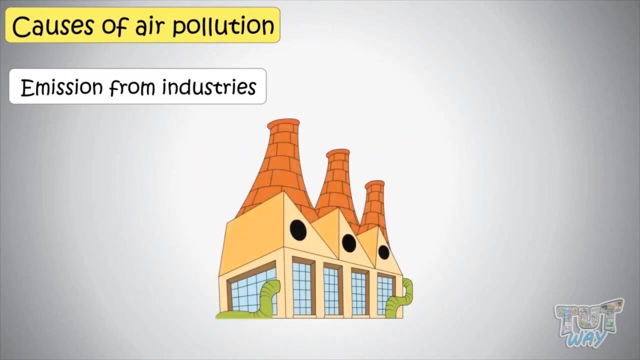 An ozone is a gas that is very harmful for our lungs. smog also reduces the visibility. we learnt a few major effects of air pollution. now let's learn what are the major causes of air pollution. emissions from industries and manufacturing activities. almost all types of industries emit a lot of smoke. that is. 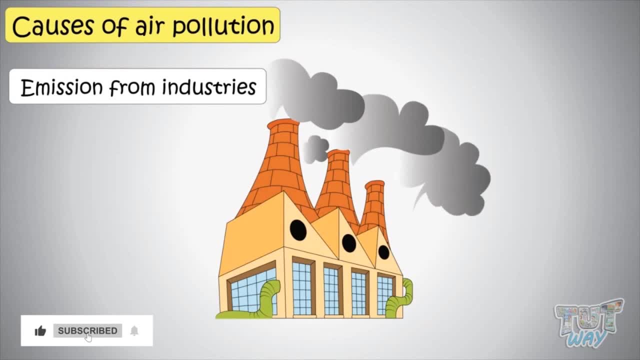 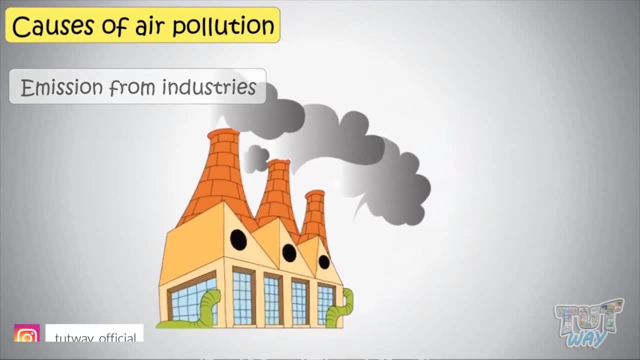 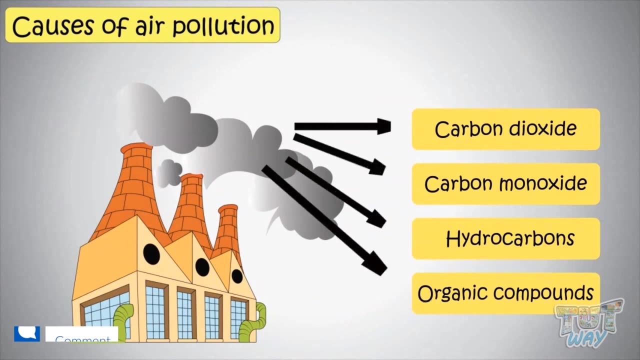 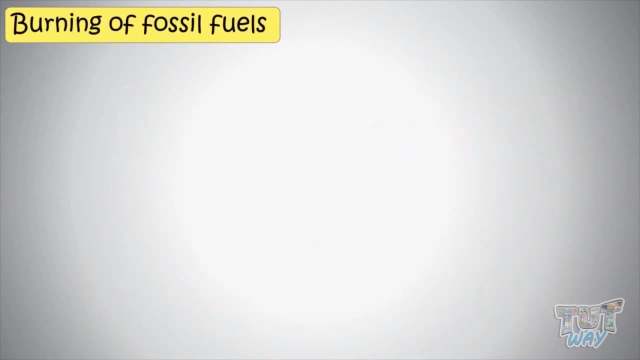 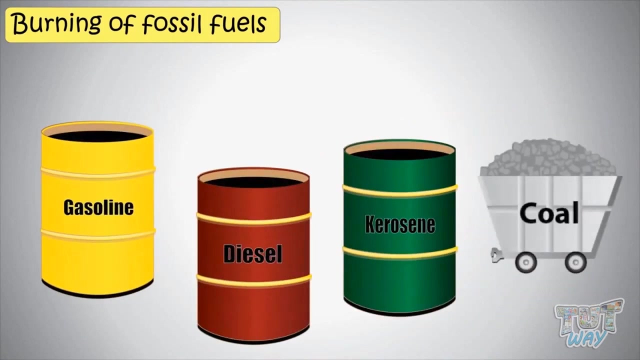 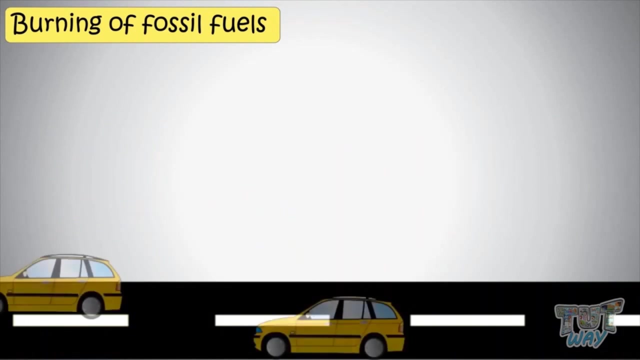 released into the atmosphere and pollutes the air. their smoke has high levels of harmful gases and particles like carbon dioxide, carbon monoxide, hydrocarbons and organic compounds that are very harmful. burning of fossil fuels- fuels like gasoline, diesel, kerosene, coal are examples of fossil fuels. all vehicles use some fossil fuel, mainly gasoline, for running. 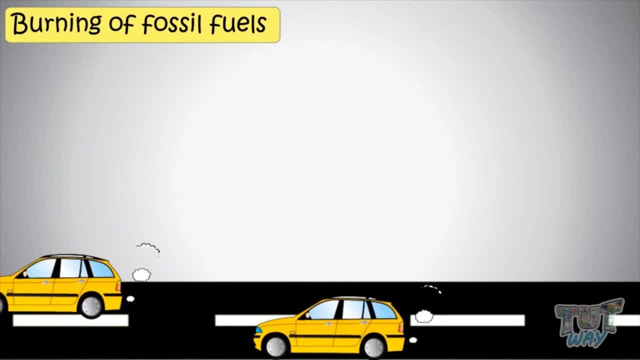 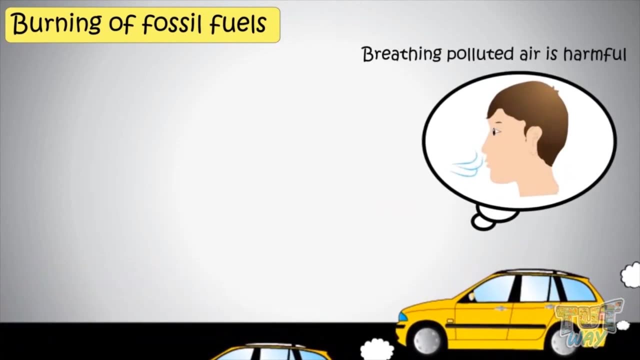 and emit a lot of smoke. that contains a lot of pollutants like carbon monoxide, oxides of nitrogen, hydrocarbons and particulate matter. carbon monoxide, oxides of nitrogen, hydrocarbons and particulate matter: on their own, they cause great harm to people who breathe them and, additionally, 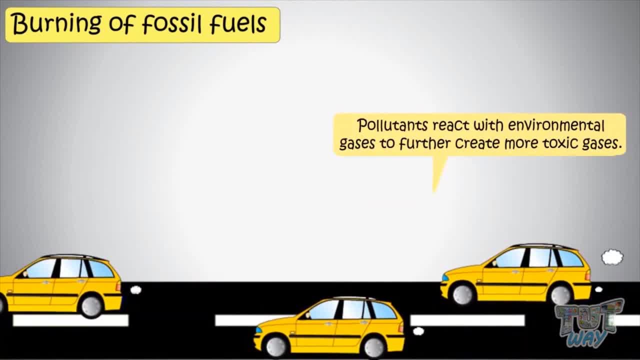 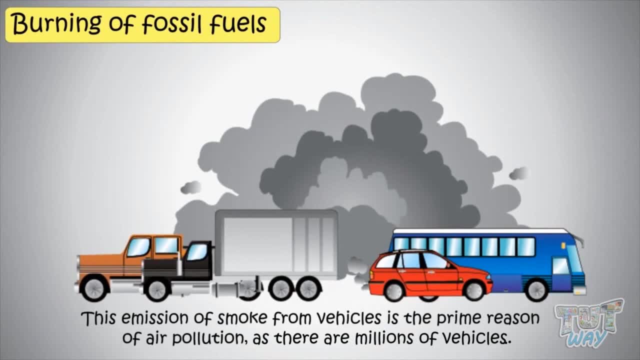 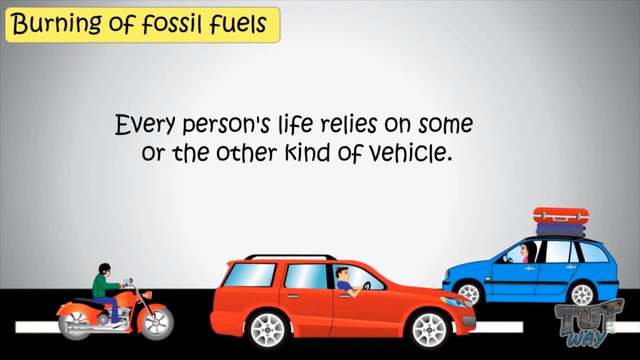 they react with the environmental gases to create further toxic gases. this emission of smoke from vehicles is a prime reason of air pollution, as our world consists of vehicles in millions, as today, every person's life relies on on some or the other kind of vehicle. Vehicles are required for transporting goods and to 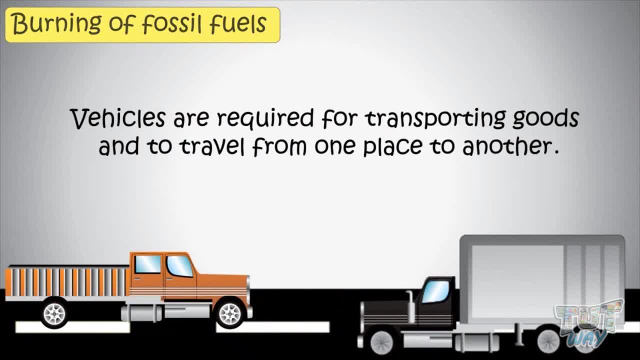 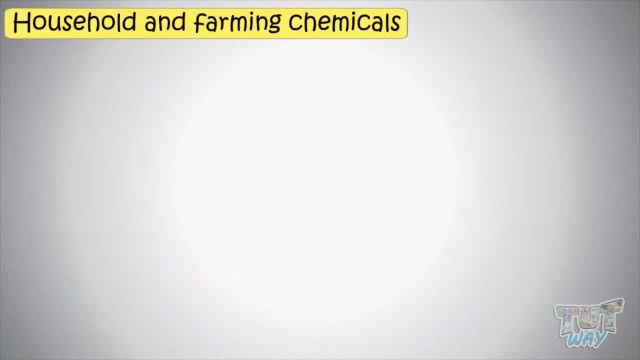 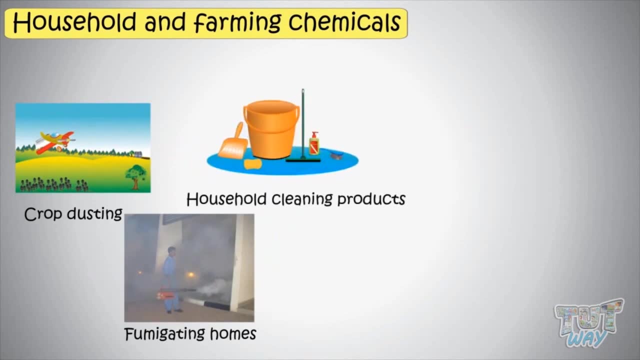 travel from one place to another, and we all need to travel. Household and farming, chemicals, Crop dusting, Fumigating homes, Household cleaning products, Painting supplies, Insecticides, Weedicides, Fertilizers- All emit harmful substances into 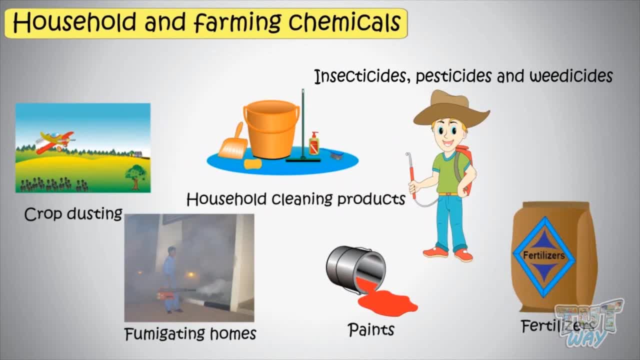 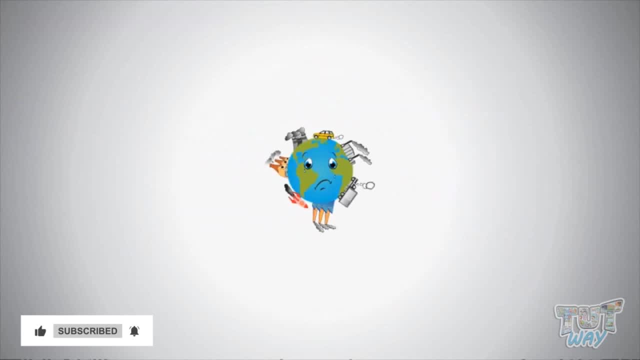 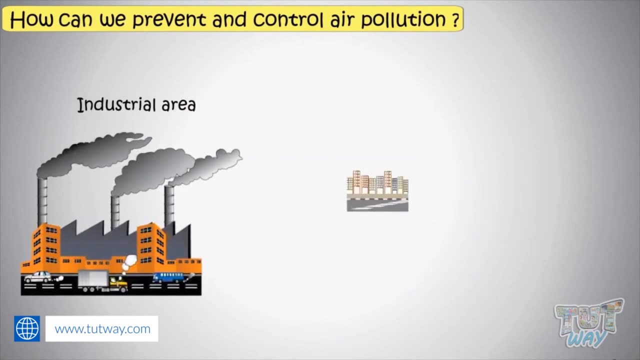 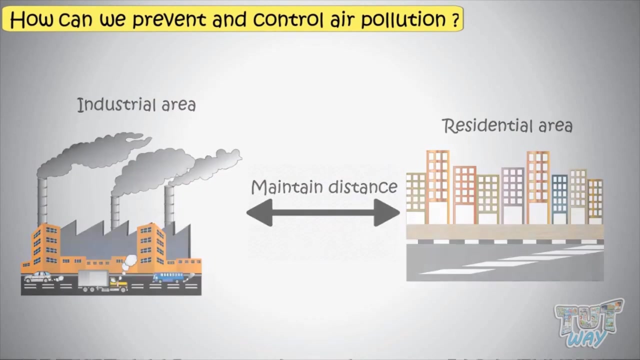 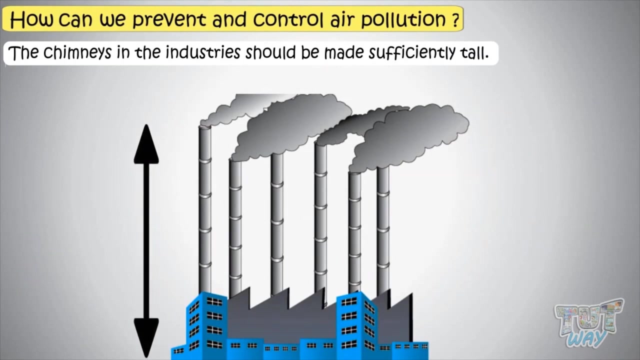 the air and cause some kind of pollution. So, kids, we learn what are the major causes of air pollution. Now let's learn how we can control air pollution. There should be sufficient distance between industrial and residential air pollution. The chimneys in the industries should be made sufficiently tall so that smoke is released as. 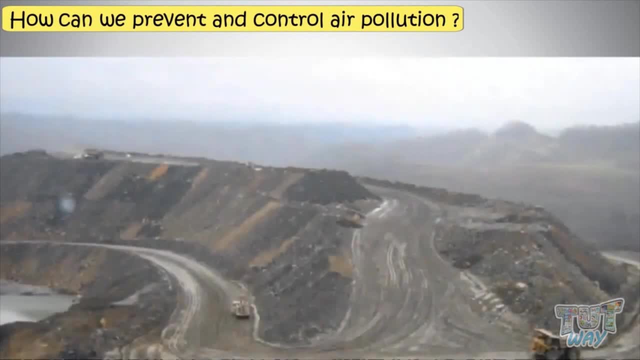 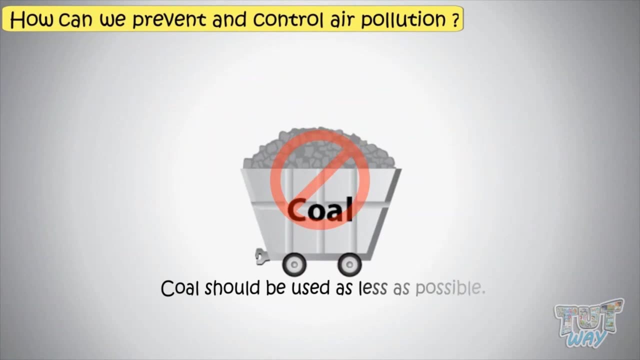 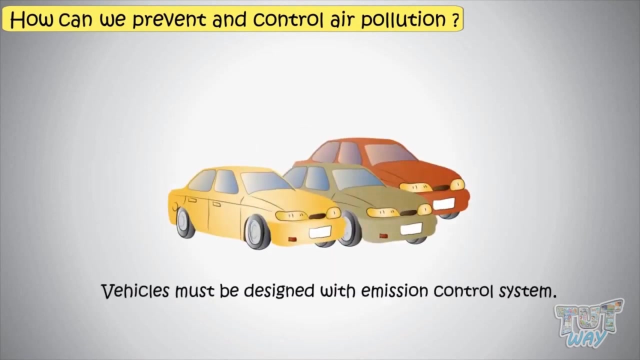 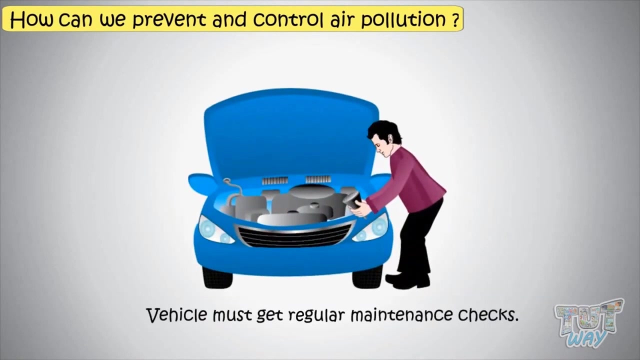 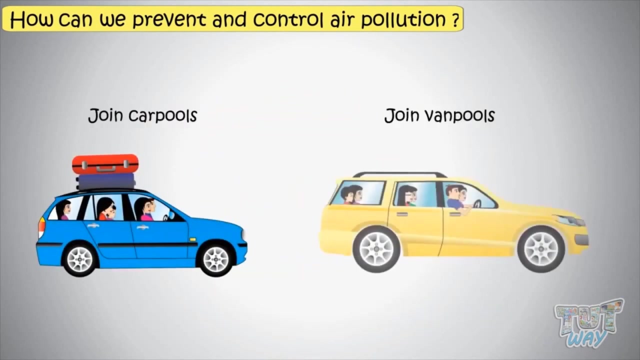 higher as possible. The mining areas should be planted with trees. Coal fuel should be used least possible. Vehicles must be designed with emission control systems. Vehicles must get regular maintenance checks. We must try to join carpools or vanpools so as to save fossil fuels. 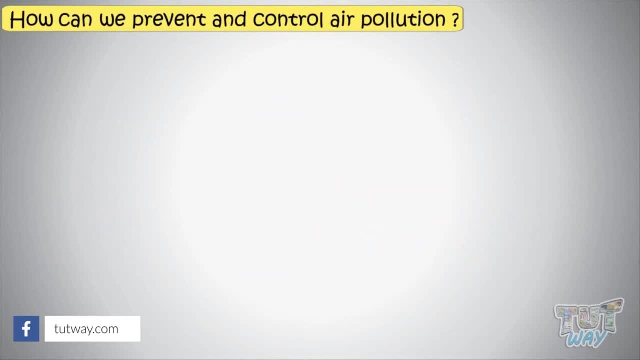 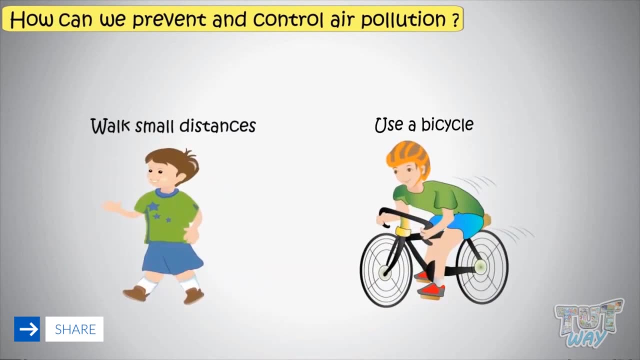 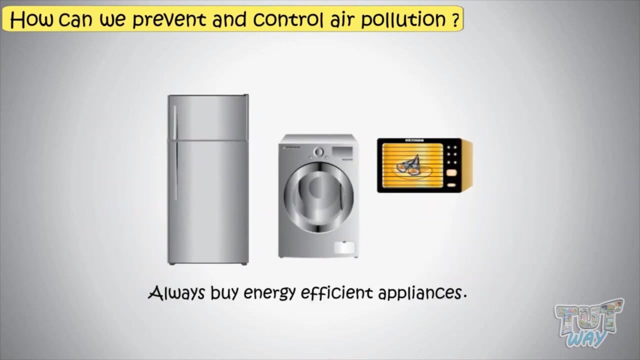 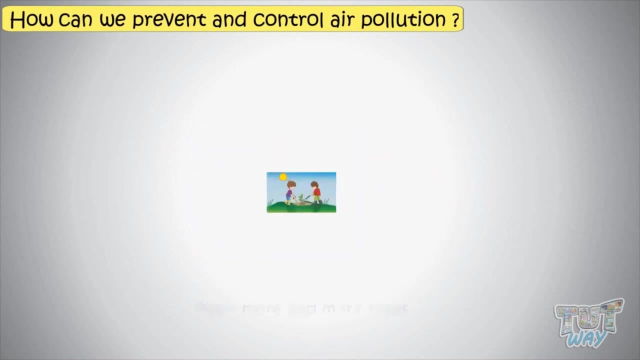 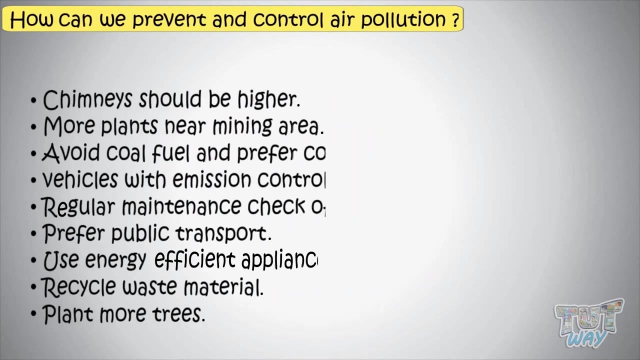 Always try to prefer public transports or walk small distances or use a bicycle. Always try to travel by street or bicycle. Always try to buy energy efficient appliances, recycle newspaper, aluminum and plastic waste. We should plant more and more trees. So, kids, these are small steps that we can take to prevent air pollution.